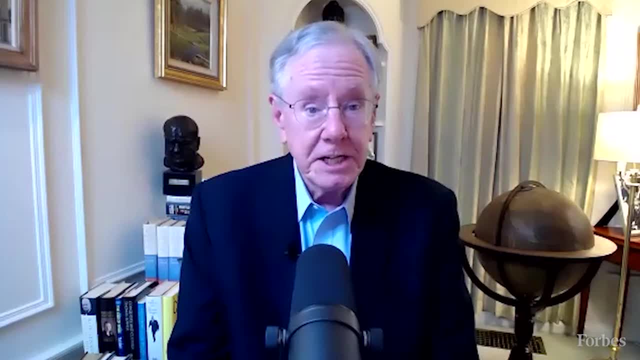 Knowing the fundamentals of our government and our history are essential for having an informed and effective citizenry. Yet shockingly few Americans know about these basics. Here's a simple way to remedy that. Hello, I'm Steve Forbes and this is What's Ahead. 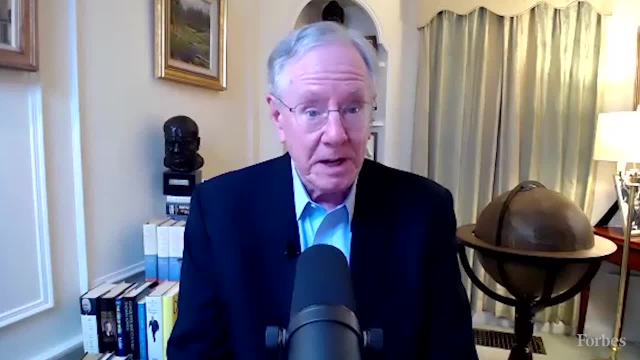 where you get the insights you need to better navigate this turbulent world. Countless Americans have been using online services to learn more about their ancestry. Yet few people today know the basics about our own country, that is, our system of government and our history, Having elementary knowledge of what makes the US tick, so to speak. 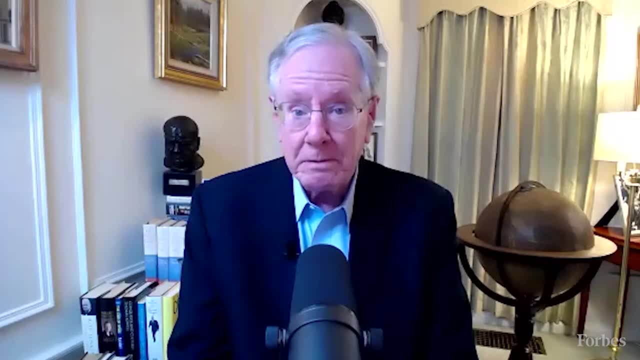 and why it has been a magnet and an inspiring example to countless numbers of people around the world for over two centuries, is important for American citizens to understand, Which is why we require those immigrants who want to become citizens to study and pass a test on our history. 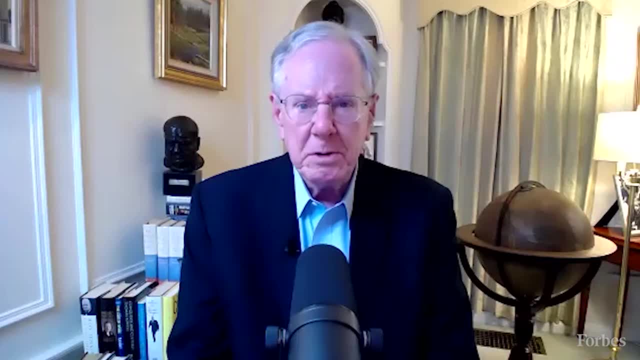 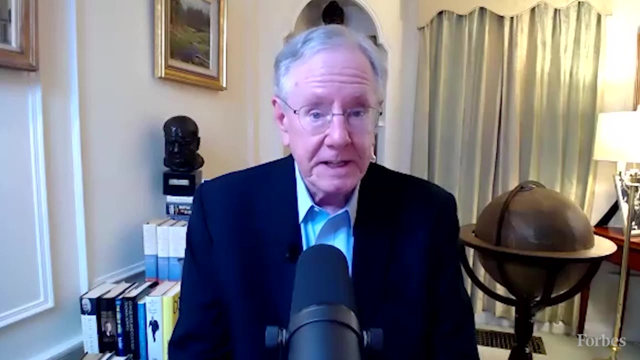 and our form of government. Yet for years, most of our schools have been derelict in teaching kids what used to be called civics- the fundamentals of the US. This abysmal ignorance is shocking, But there is a simple solution: Have our schools teach civics based on the naturalization test. 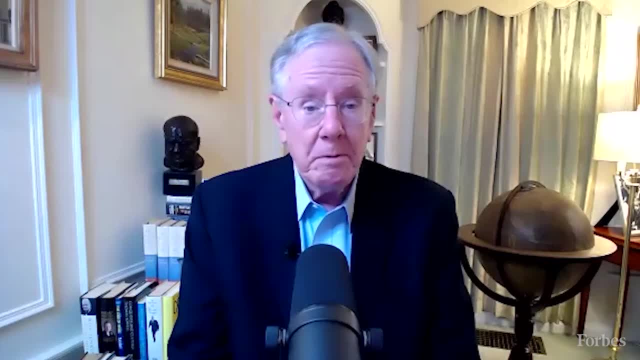 given to immigrants who want to become US citizens. Before gaining citizenship, an immigrant must learn the essentials of our form of government and the essentials of our history. That can't be helped. A candidate has to study and absorb the answers to 100 questions. This person will be asked 10 of. 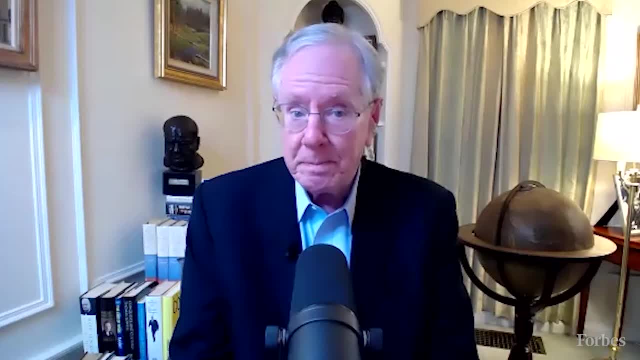 them and must get at least 6 of them right to gain citizenship. Areas and questions for this naturalization test include principles of American democracy, such as: what does the Constitution do? What are one of the rights protected by the First Amendment? What is the? 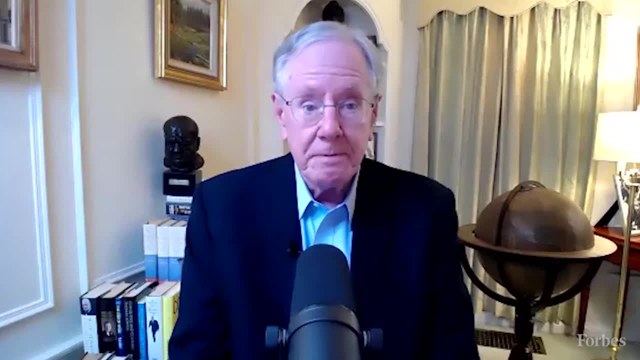 Declaration of Independence. What stops one branch of government from becoming too powerful? What are the two parts of the US Congress? What are one of the four amendments to the Constitution about who can vote? There are history questions such as what is one thing?